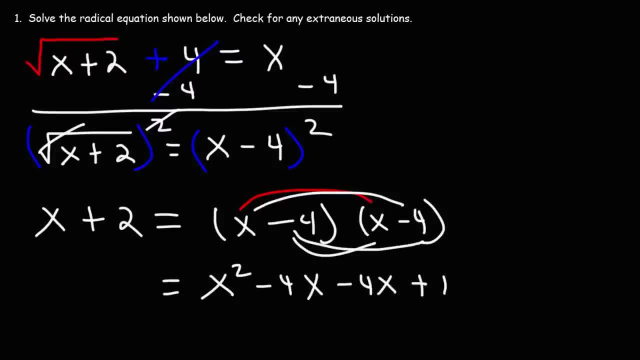 and then negative 4 times negative 4, positive 16.. So now let's go ahead and combine like terms on the right side, So we can combine negative 4x with another one, and that's going to add up to negative 8x, and so that's what we have at the moment. Now in 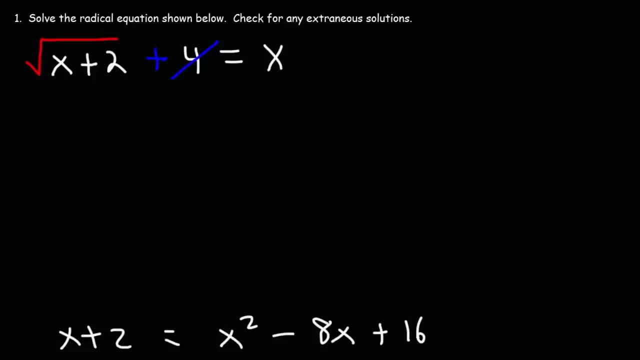 order to solve for the value of x, we need to move everything from the left side to the right side. So if we move x to the other side, this is going to be negative x, Negative 8x and negative x. that's a negative 9x. If we move the 2 to the other side, it's going 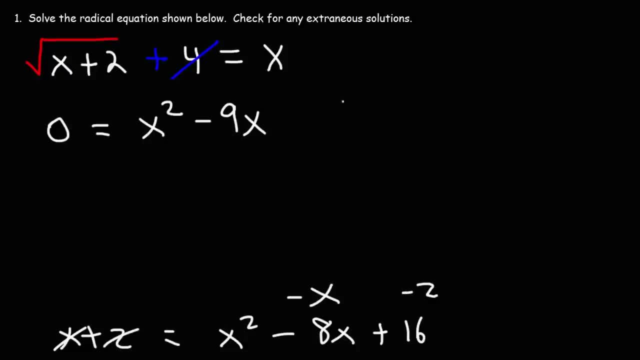 to be negative 2. on that side, 16 minus 2, that's going to be positive 14.. So now, at this point we need to factor what two numbers multiply to positive 14, but add to negative 9x. We have 1 and 14 and 2 and 7.. Now 0, 2 times 7. 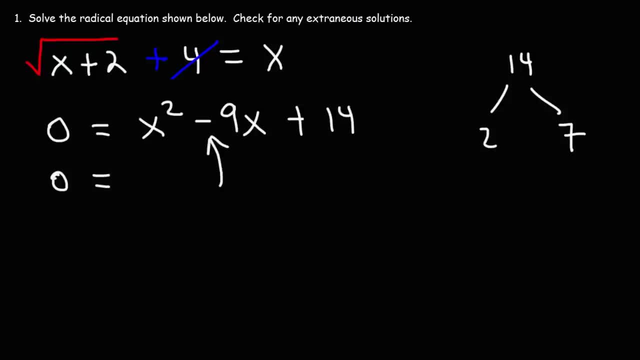 that's positive 14, but in order for it to add up to negative 9x, we need both negative 2 and negative 7. negative 2 plus negative 7 will add up to negative 9, but will still multiply to positive 14, so we can write this as X minus 2 times. 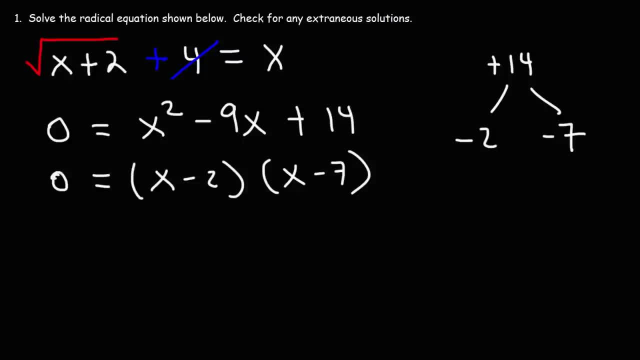 X minus 7. now, using the zero product property rule, we can set each factor equal to 0, because 0 times anything is 0. so we could set X minus 2 equal to 0 and X minus 7 equal to 0. add in 2 to both sides. we get that X is equal to. 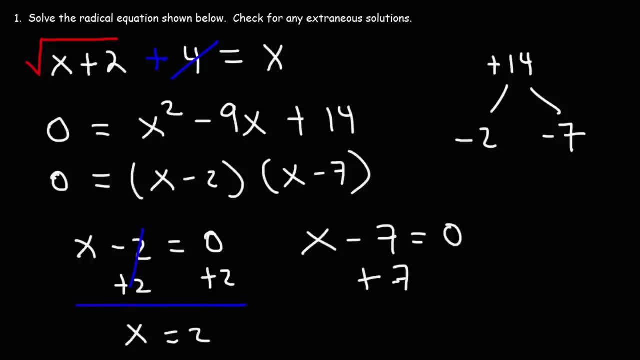 positive 2, and then for the other one we just gotta add 7 to both sides and we get: X is equal to positive 7. so those are the two solutions that we have for this radical equation. the question is which one is extraneous and which one is the real solution. so we 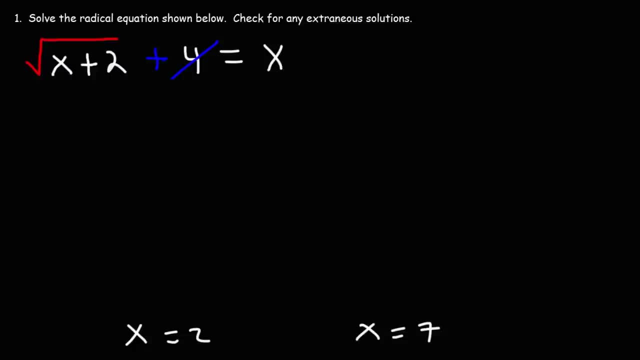 need to test them both to find the answer. let's start with this one X equals 2, so everywhere we see an X value, we're going to replace it with 2. so now 2 plus 2 is 4. the square root of 4 is 2, and 2 plus 4 is 6. now 6 does not equal 2, so therefore, 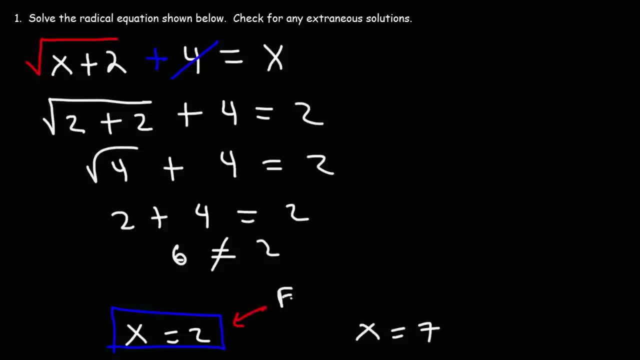 this solution didn't work for the original equation, so this is an extraneous solution. now let's try the other solution. X equals 7. let's check to see if it's extraneous. so let's replace X with 7. 7 plus 2 is 9. the square root of 9 is 3, 3 plus 4 is 7 and 7 equals 7. so this is: 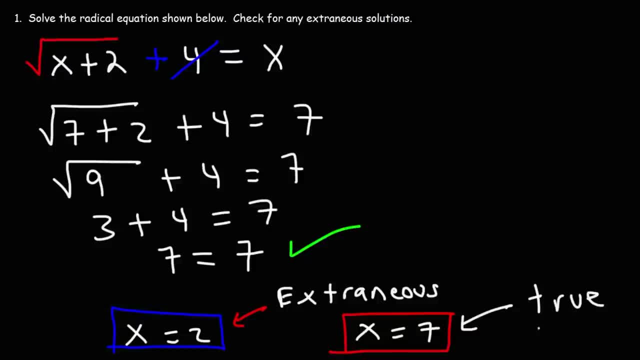 the true solution, the solution that works in the original equation. so now you know how to identify or how to check for any extraneous solution. the key is just to take that solution, plug it into the original equation and see if it works for the original equation. if not, that. 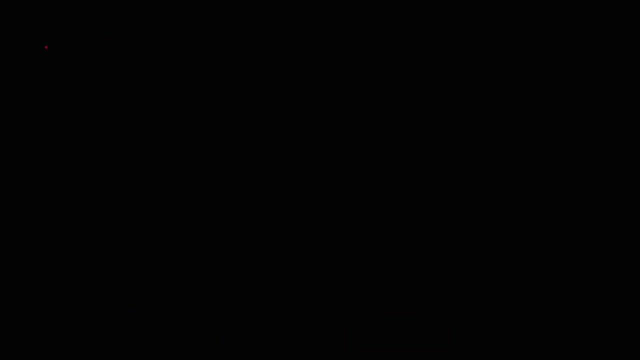 solution is extraneous. now let's try another example for the sake of practice. so let's say we have the square root of 2x and that's equal to X minus 4. so feel free to pause the video and work on this example problem check for. 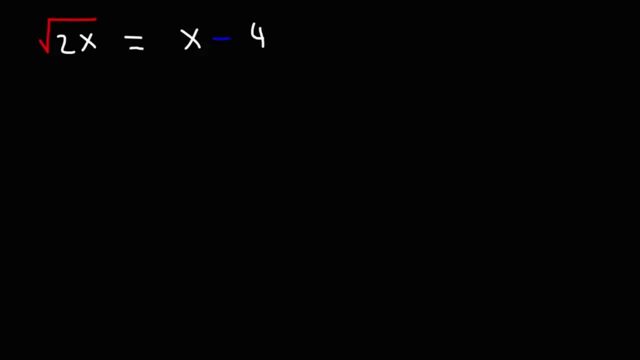 any extraneous solutions now. in order to solve for X, the first thing we need to do is take the square of both sides, just like before. the square and the square root will cancel. so on the left side we'll just get 2x. on the right side we need to expand this expression: x minus 4 squared is 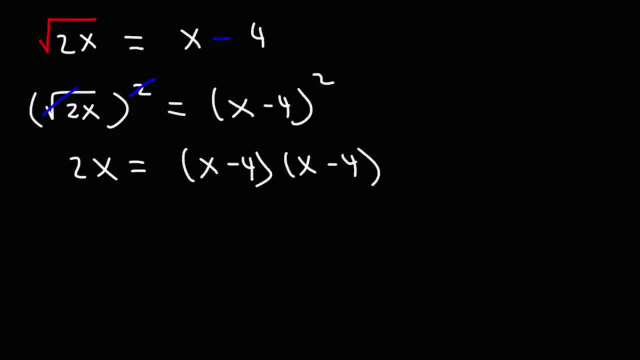 equivalent to x minus 4 times x minus 4 x times x is x squared X times negative 4. that's negative 4x. this will be negative 4x as well, and that's going to be positive 16. so So, combining like terms on the right side, we're going to have x squared minus 8x plus 16.. 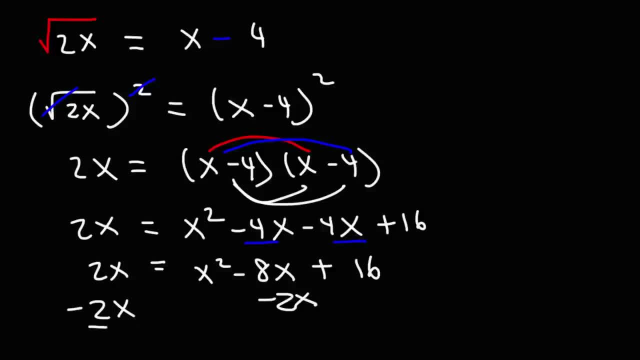 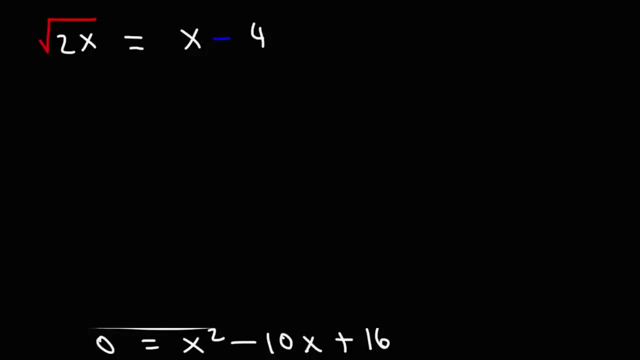 Now let's subtract both sides by 2x, So we'll have: 0 is equal to x squared minus 10x plus 16.. So now we need to factor: What are two numbers that multiply to 16, that add to negative 10?? 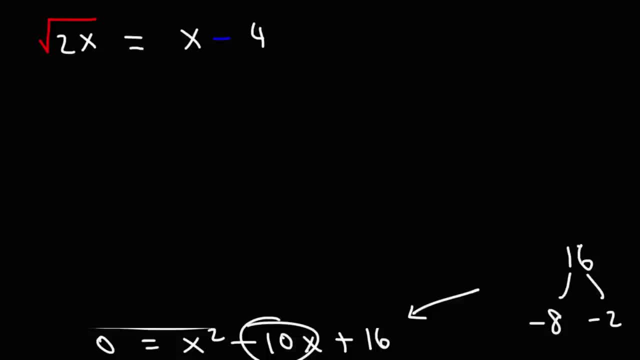 So this is going to be negative 8 and negative 2.. Negative 8 plus negative 2 is negative 10, but they multiply to positive 16.. So we can factor this trinomial as x minus 8 times x minus 2.. 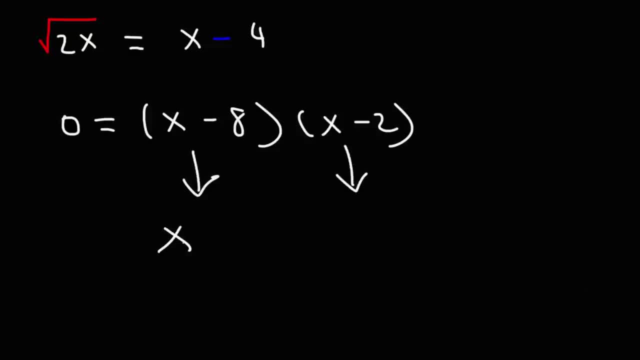 Now, using the zero product property, we're going to get the solutions: x is equal to 8. Let me run that, Let me run that, Let me write it below here. And x is equal to 2.. Now let's see which of these, if any, is extraneous. 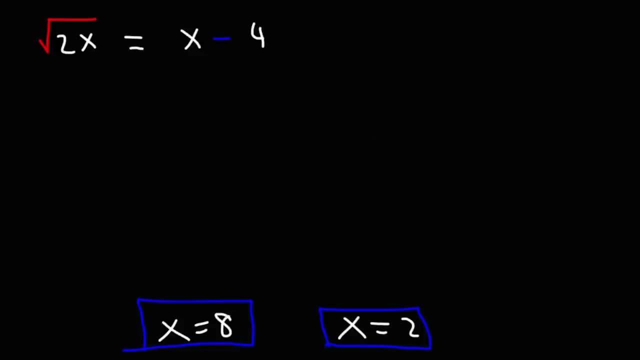 So let's start with the first one. Let's plug in: x equals 8 to the original equation. So we're going to replace x with 8. And we'll have this 2 times 8 is 16.. 8 minus 4 is 4..